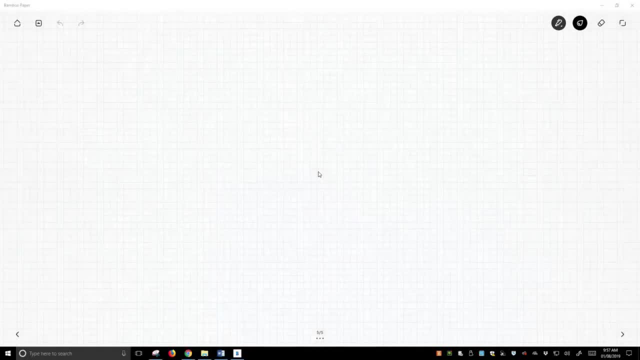 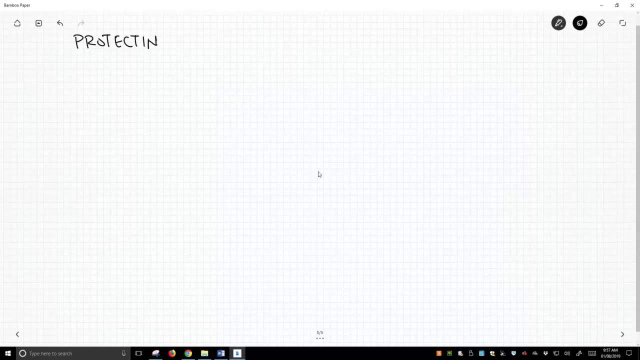 Anytime people discuss acetyls and ketals, you quickly bump into a topic called protecting groups. Protecting groups- Okay, you are actually very familiar with this idea. Anybody who's done painting in a house understands this. and even if you haven't done painting, you've seen. 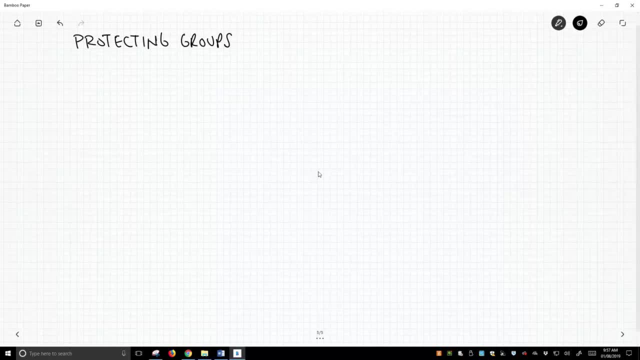 commercials with people painting the whole nine yards. So let's say we want to paint a wall, This is our wall, and what you oftentimes see on a wall is trim at the top and the bottom. Maybe you have some crown molding, Maybe you have some floor trim, but there's some kind of trim and here's. 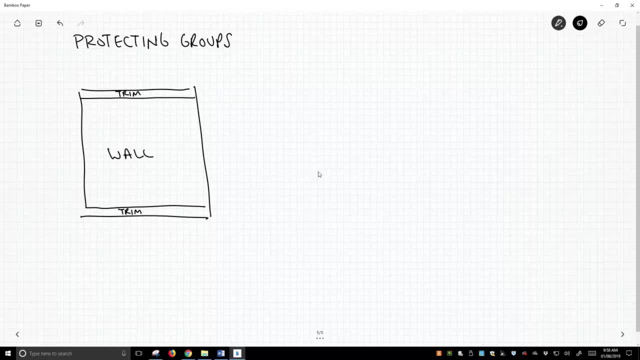 your wall and you want to paint this wall. Now, if you're not a really skilled painter- and I am not a really skilled painter- if I wanted to do this, I would need to put masking tape on the trim, And taping things is a hassle, but I'd have to do it. I'd have to put tape over the edge of the trim. 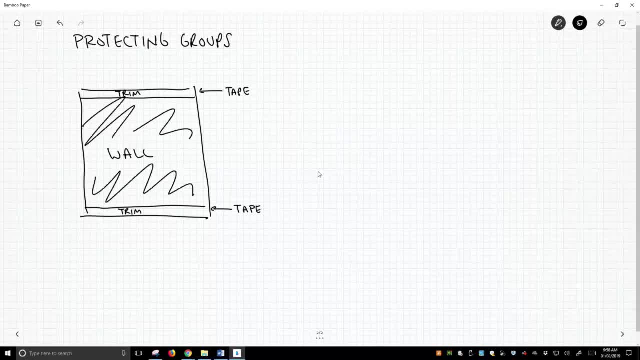 so that I could freely paint this wall and not make a mess of my trim, which is probably going to be a different color. Then, once I'm done, I remove the tape. So to paint the wall- that's my goal. I'm going to need three steps. I'm going to need to tape. 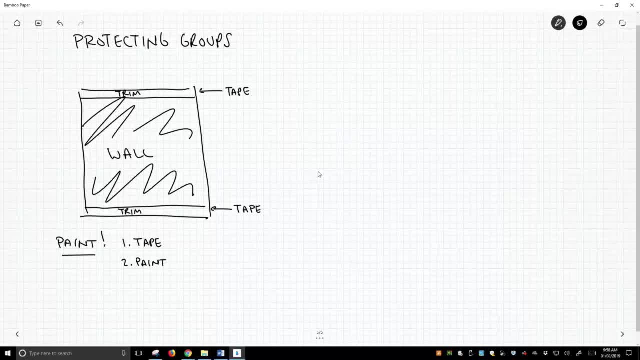 then I'm going to paint the wall and then I've got to remove the tape And you might say this is kind of a waste of time because that doesn't help me achieve my goal, which is paint the wall. But if I want to do a good job, I've got to protect the trim. 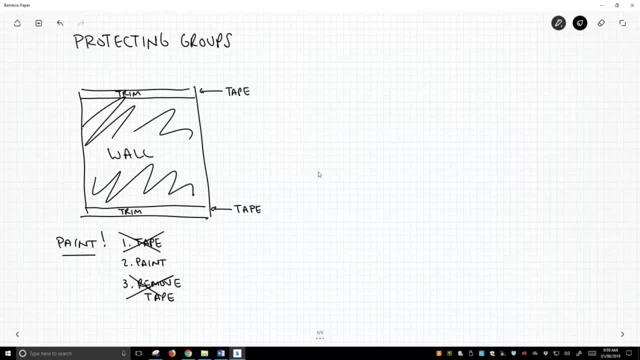 so I don't get paint all over the place. If you're a professional painter, maybe you don't have to trim. It's a whole other story, But for me I have to have inefficiency, this extra taping, and remove the tape to get the job done. The same thing happens in chemistry. So let's say we have a molecule. 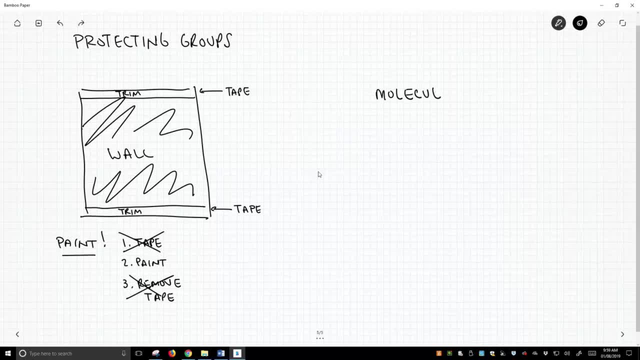 and it's just going to be our jelly bean molecule and we have a functional group out here and we have a functional group out here among other things that might be in our molecule. Let's say we want to do a reaction on the function of the left hand functional group.